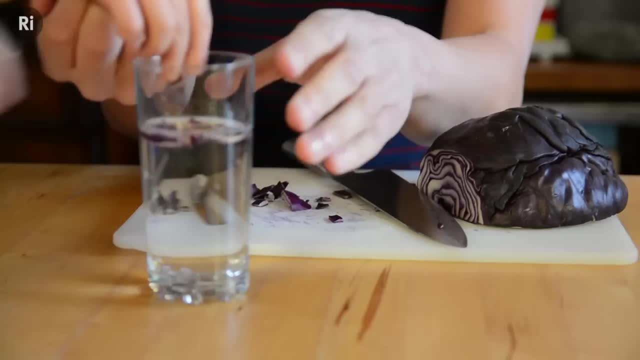 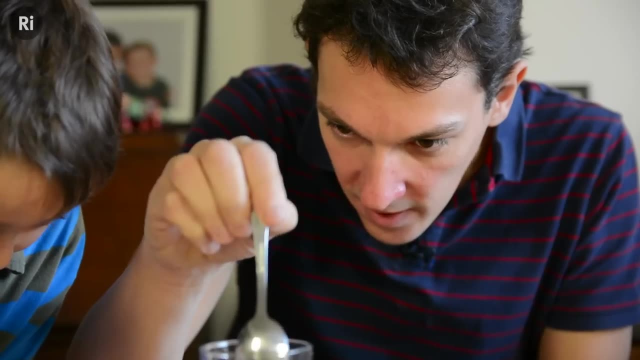 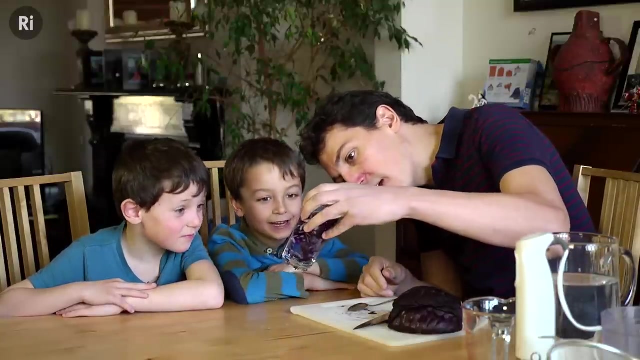 Oi, Cabbage, Right, okay, Oh no, there's tons of cabbage. It's getting dark Blue. Why is it going blue? Because the cabbage-like colour is making it blue. It's taking it down. So do you think the cabbage colour is coming out of the cabbage and going into the water? 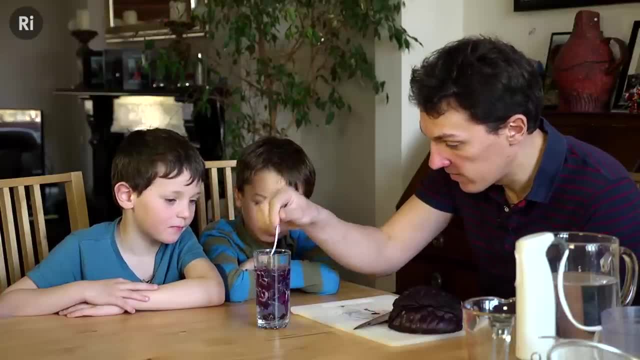 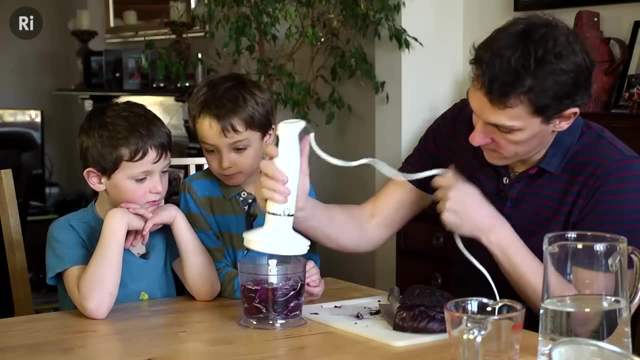 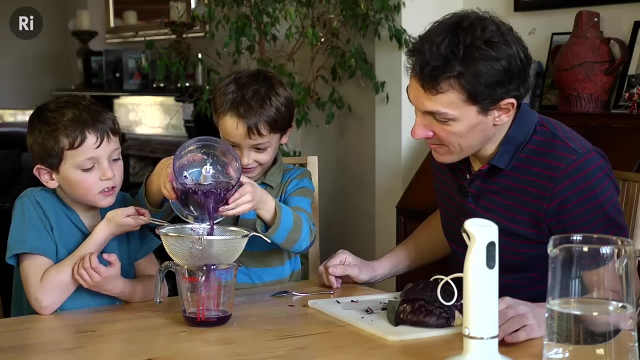 Yeah, So you can do some really fun things with this coloured water, but we need to make loads more. This kind of cabbage is red because it contains chemicals called anthocyanins. Blitzing the cabbage in water, lets us extract those chemicals and use them for our experiments. 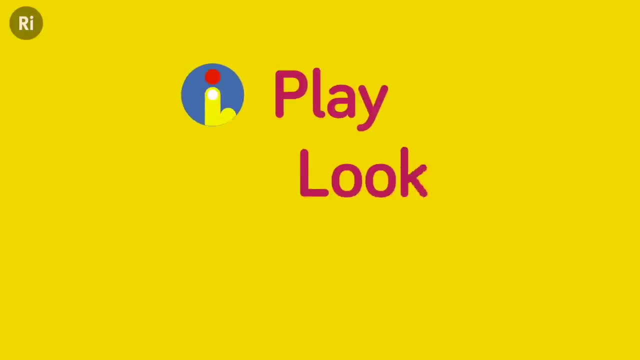 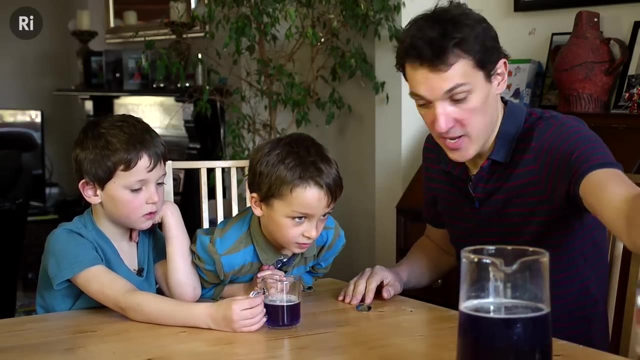 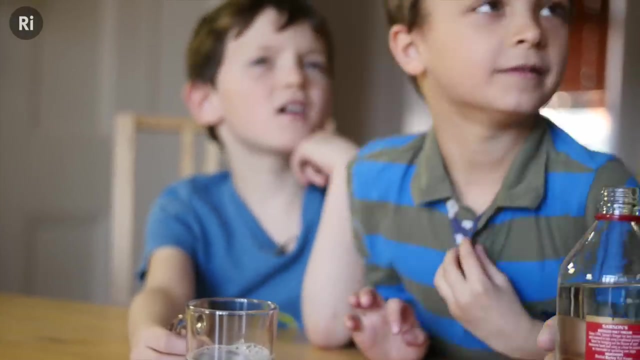 Right, we're going to do some science now with this. I'm going to get some vinegar, I'm going to pour it in there. What do you think might happen? Change, a little bit of colour. A little bit of colour. What do you think, Tom? 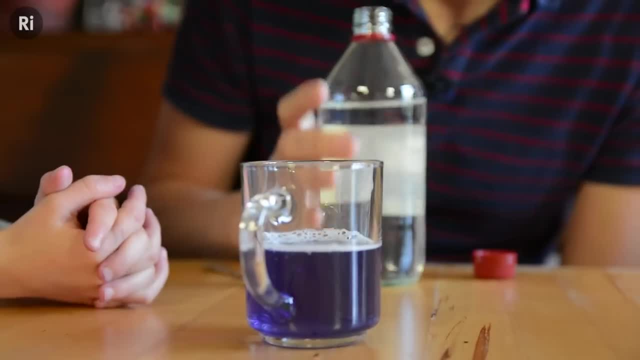 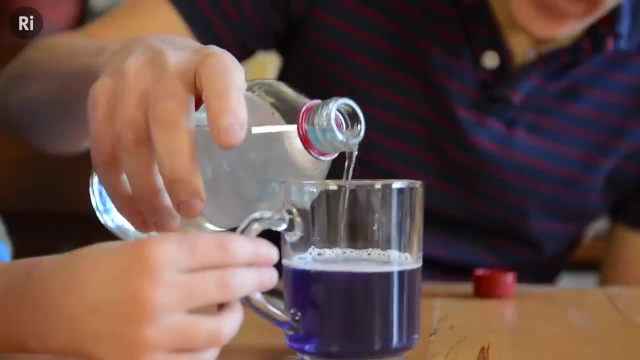 It'll explode. Maybe it will explode, Okay, so look carefully while I pour this, Look what happens. It's going to change colour. I think it is going to change colour. That's good, I can smell the vinegar Cool. 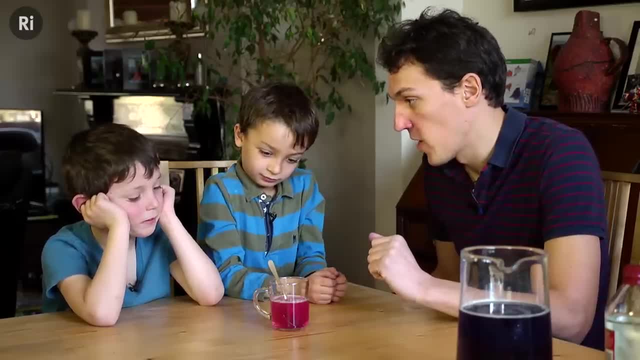 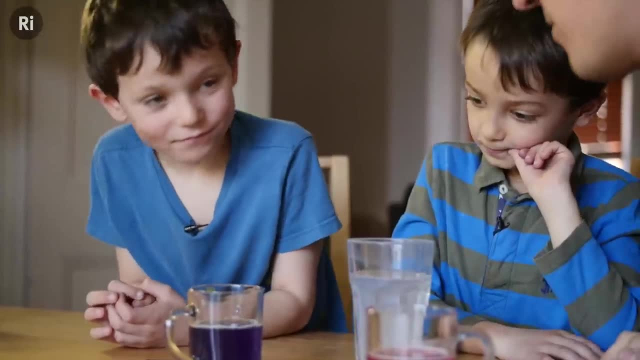 So this cabbage water kind of changes colour in a slightly strange way, doesn't it? So should we see if it changes colour with other things? Yeah, This is actually bicarbonate of soda. What do you think might happen this time? It's going to go all fizzy. 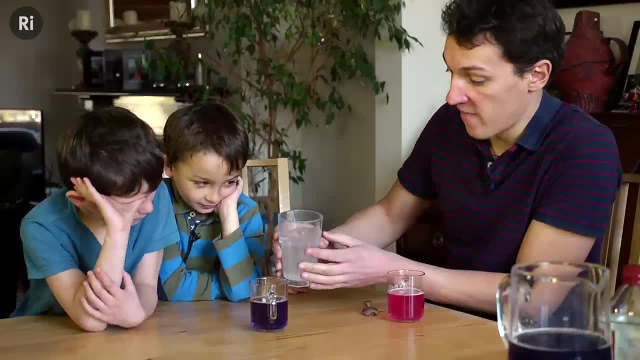 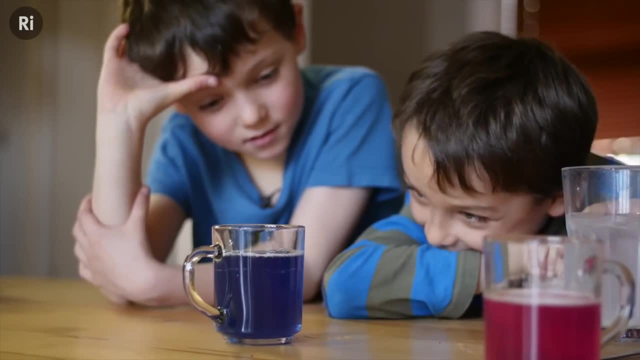 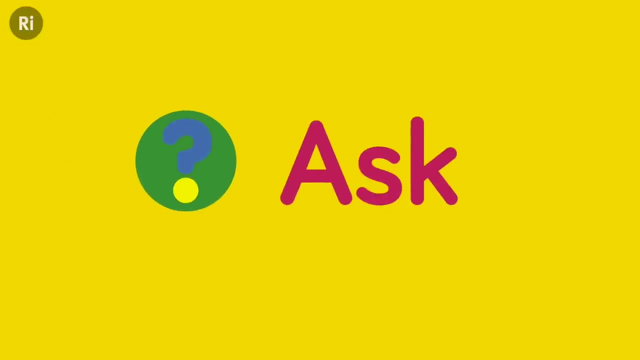 Me too, Sorry. I think it's going to go all fizzy. So watch carefully what happens again. I know now. I knew it was going to turn blue. Look at that. No, you didn't. So let's try some fizzy water, yeah. 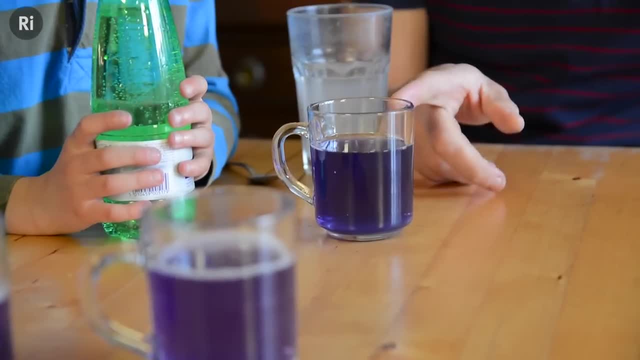 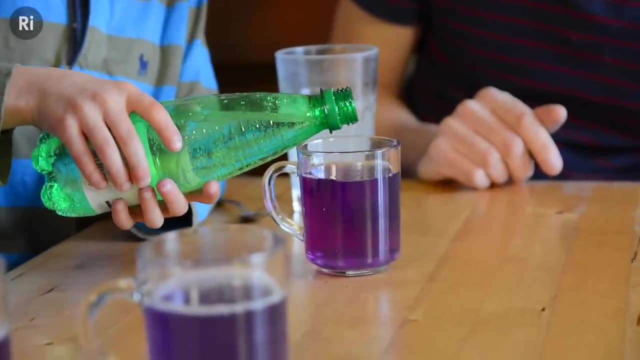 Yeah, Yeah. So what colour, guys, do you think this is going to go this time? A different colour completely. Yeah, Me too, Because it's a different thing. What's going on? Oh Okay, keep pouring. I think it's going to turn pink. 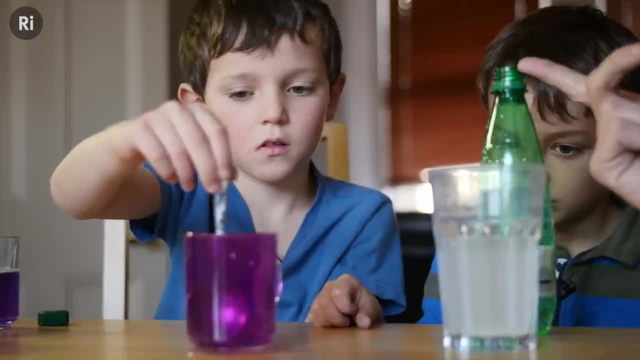 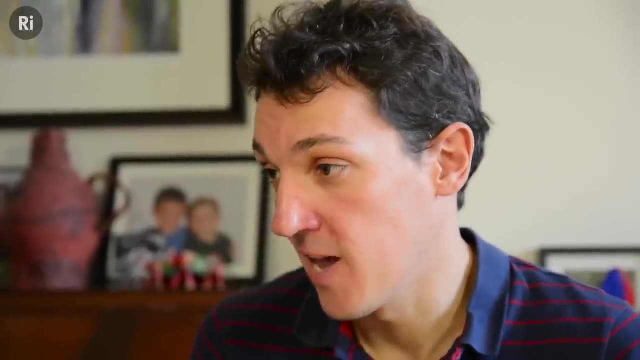 Keep pouring. It's going pinker. Is the water more like the vinegar or more like the bicarbonate of soda? More like the vinegar? Yeah, So there's something in common with the fizzy water and the vinegar. It's fun to just look at all the colour changes that you can get with this cabbage juice.